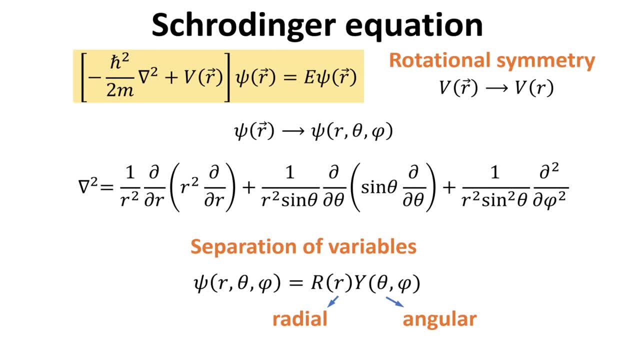 We shall begin with looking for solution that are separable into products of functions R and Y, where R is only a function of R and Y is only a function of theta and phi. We shall insert this new separable form of the wave function into the Schrodinger equation. 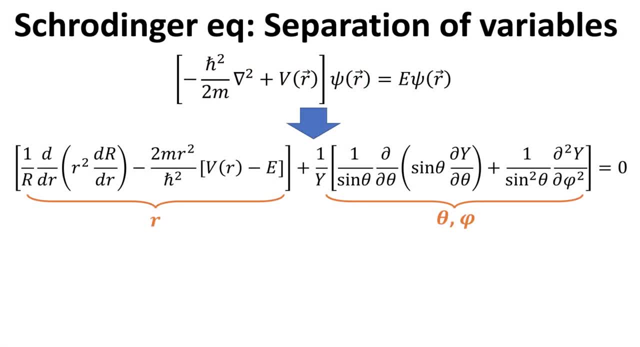 After some manipulation and dividing the equation throughout by the wavefunction and multiplying by the constant minus 2rm square divide by h-bar square, we obtain the following as shown. We see that the expressions within the first square bracket depends only on the coordinate. 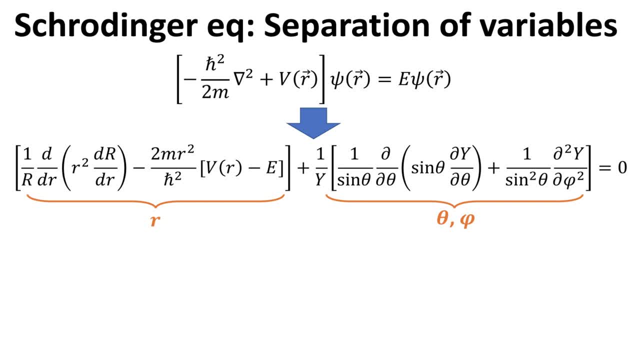 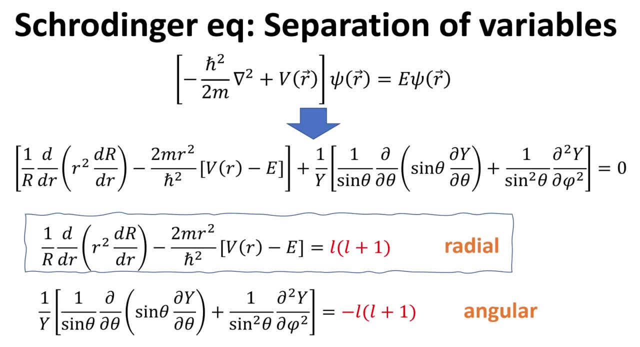 r, while the expressions in the second square bracket depends on theta and phi only. Hence these two expressions must each be a constant. for the equality to be satisfied, We shall let the constant be L multiply by L plus 1, for reason that will become apparent. 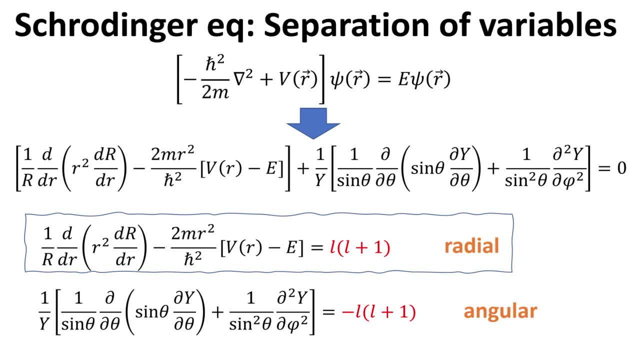 later. The first equation is the radial equation, which depends on the Coulomb potential energy term, whose solutions will be presented in this video. The second equation is the angular equation, whose solutions give us the spherical harmonics y, which we have already presented. 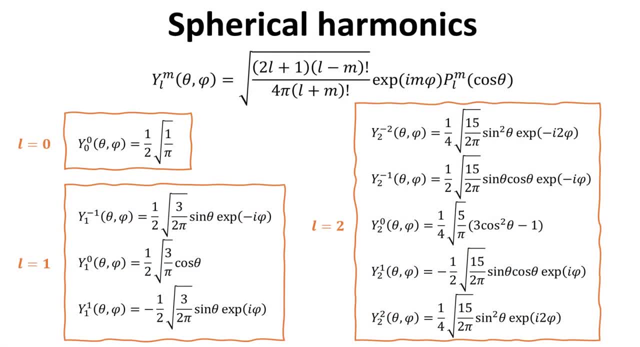 For your convenience we show here again the explicit expressions of the spherical harmonics function y for L equals to 0,, 1 and 2, as we shall see later when we solved for the hydrogen atom. These are the L states that are most relevant. 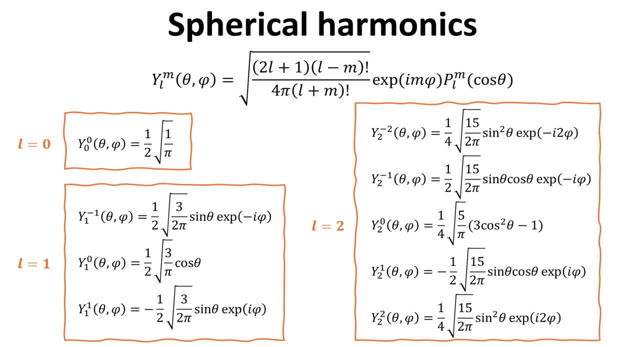 For each index L, we access only M from minus L to plus L. Thus, for L equals to 0,, we have only M equals to 0.. For L equals to 1,, we have M of minus 1, 0 and plus 1.. 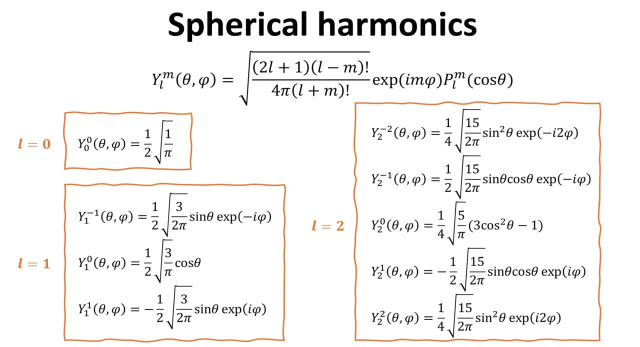 For L equals to 2,. we have M equals to minus 2, minus 1,, 0,, 1 and 2.. Thus one spherical harmonics for L equals 0,, three spherical harmonics for L equals 1, and five spherical harmonics for L equals 2.. 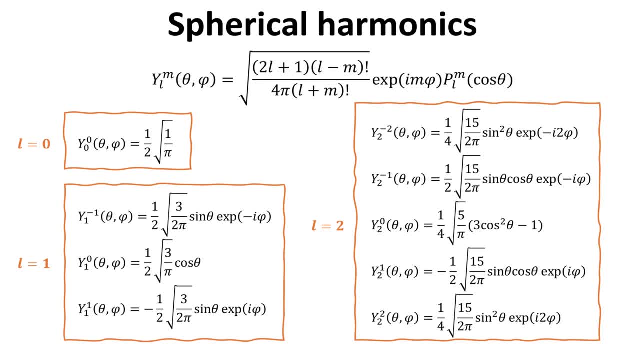 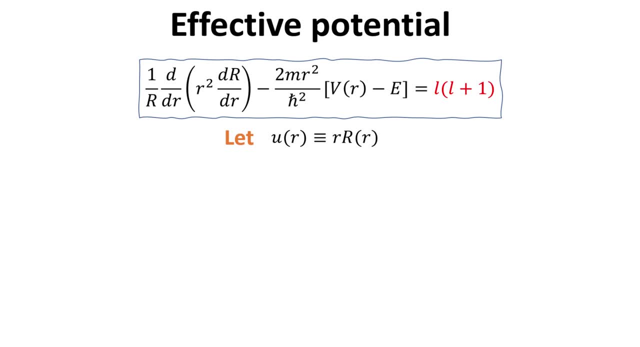 We see that these spherical harmonics are complex functions due to the complex exponential functions. Now back to the radial equation. Our first task is to tidy up this equation. We define a new function, U, as a product of the radial coordinate R and the function 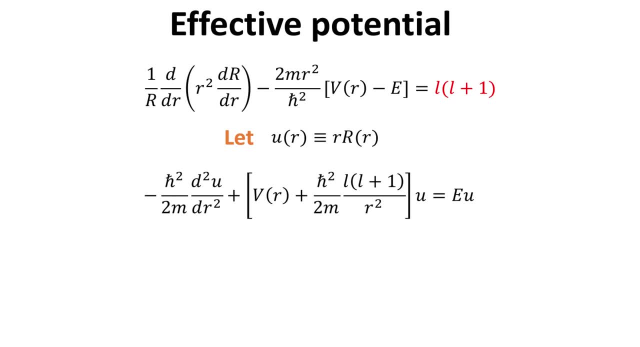 R. Substituting this new function U into the radial equation, we arrive at a new second-order differential equation for the function U. We see that this new radial equation has the same form as the Schrodinger equation. if we define a new effective potential, as shown. 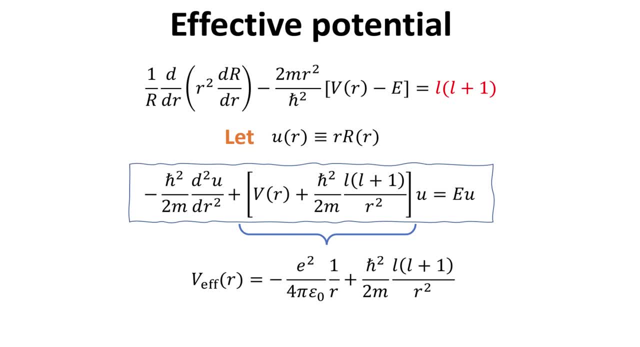 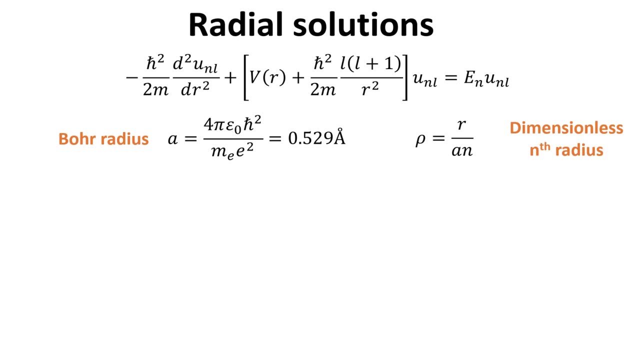 Thus this amounts to solving a one-dimensional Schrodinger equation. Of course, this can be solved very easily numerically. Luckily, it is also possible to solve this radial equation analytically. In this video, we shall not be bogged down with the math of deriving its solutions, as 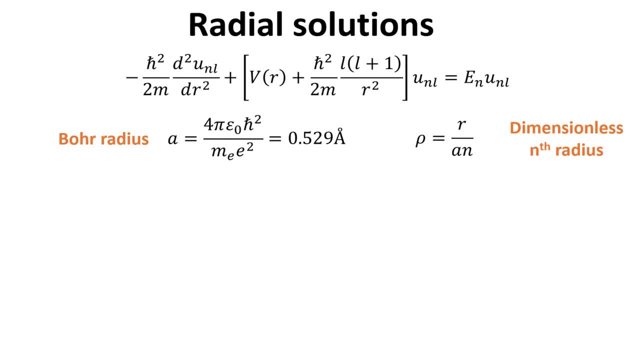 this can be found in most textbooks. Instead, we will just present its solutions and discuss the form and shape of these wave functions. First, we note that the energies are discrete and are denoted by the quantum number n. The wave functions U depends on the quantum number L and n. 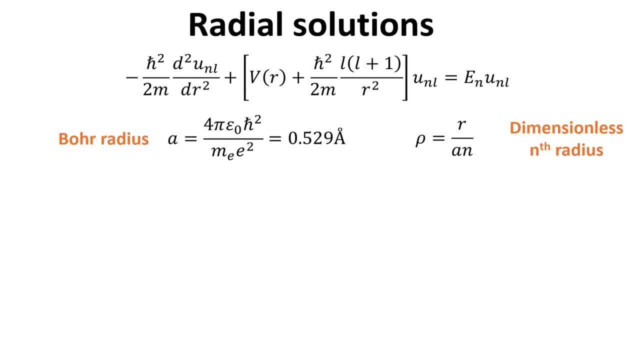 We first define the Bohr radius, defined as shown in terms of universal constants. It is about half an angstrom. We also define a new function, U, as a product of the radial coordinate R and the function R. We also define a new function, U, as defined in terms of universal constants. 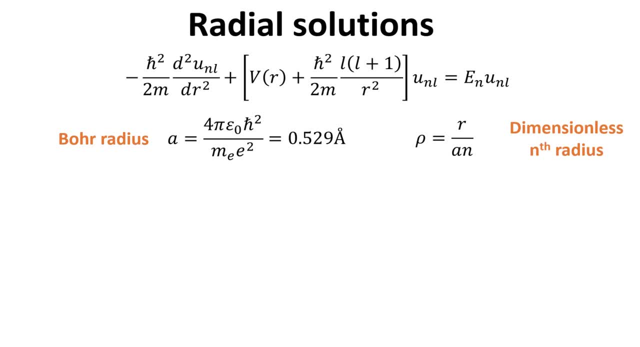 We also define a new function R as a product of the radial coordinate R and R. We also define a new function R as a fourth function and a fifth function, and this will define the second function, U, as defined in terms of universal constants. 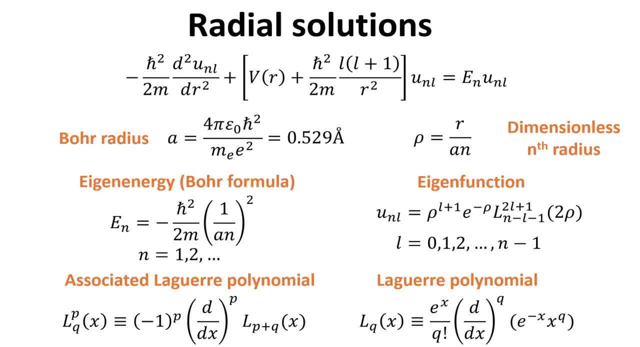 The eigen-energy En is given as follows: where n is an integer that runs from 1,, 2, and so on. This is also known as the Bohr formula, first proposed by Niel Bohr before quantum mechanics or Schrodinger equation even existed. 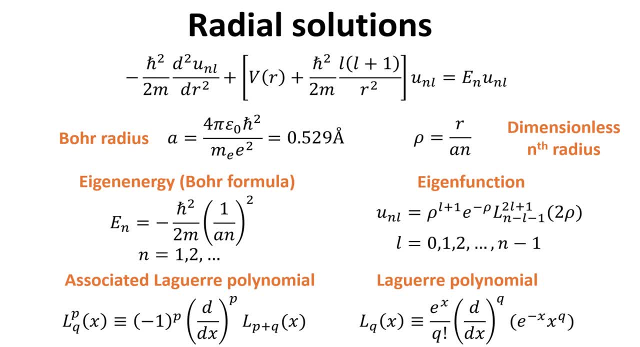 The eigenfunction is given as follows In terms of the associated Laguerre polymorphism, Laguerre polynomials and the Laguerre polynomials, The eigenfunction u are labeled by the quantum numbers n and l, where l runs from 0,, 1,, 2 to n minus 1.. Do not be scared by these mathematical. 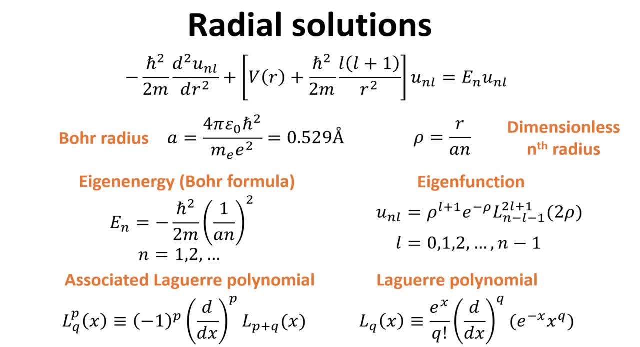 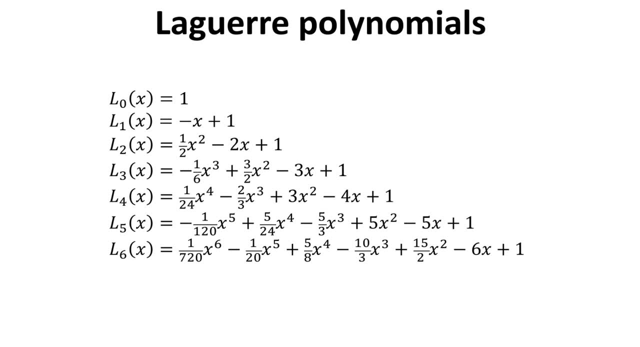 expressions. We will clean them up substantially in what follows. As the name implies, the Laguerre polynomials are just polynomials. We list the first half dozen of these polynomials here. You do not need to worry about these. I just list them here for your convenience. 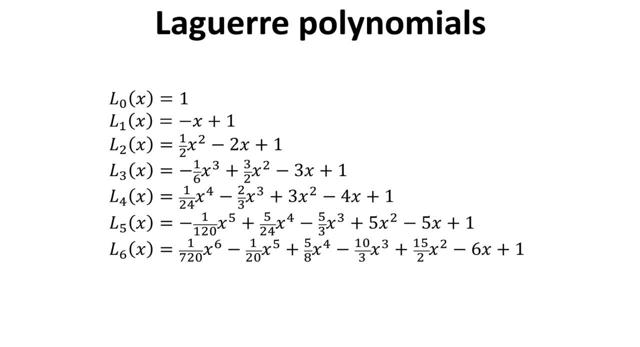 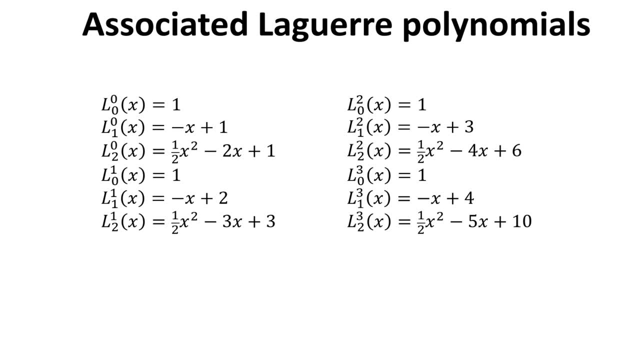 Remember the slides can be downloaded from the YouTube description link below. The associated Laguerre polynomials are also listed here for the first dozen that we will be using in this video. As you see, these are very simple polynomial functions. The radial function of the Laguerre polynomials is called the Laguerre polynomials. 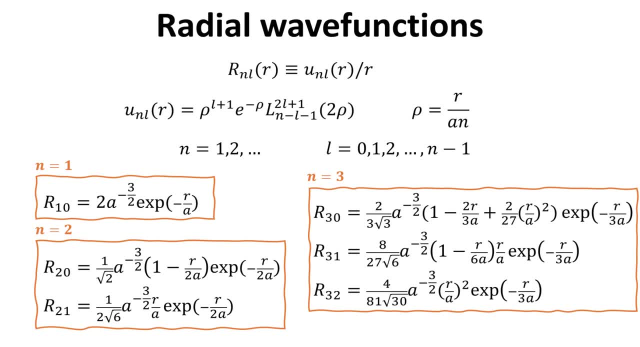 The radial function of the Laguerre polynomials is called the Laguerre polynomials. The radial wave functions r can be obtained from the function u. We list here the radial functions associated with the first, second and third energy levels denoted by: n equals to 1,. 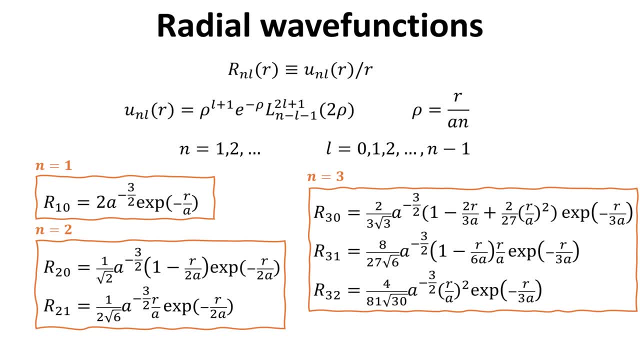 2 and 3,. as shown, The subscript for r contains two numbers: the quantum number, n and l. For n equals 1, we have only one radial function, with l equals 0.. For n equals 2,, we have two. 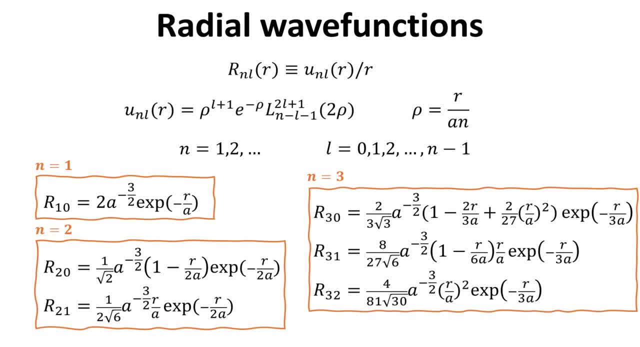 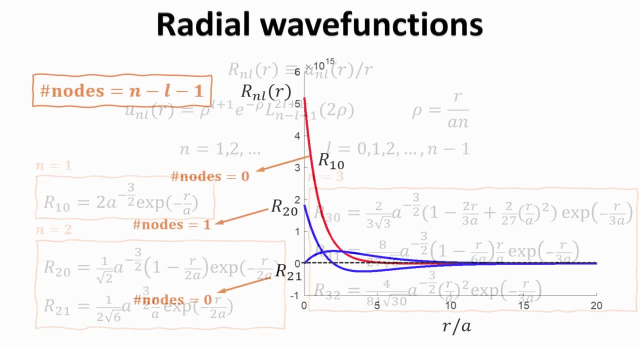 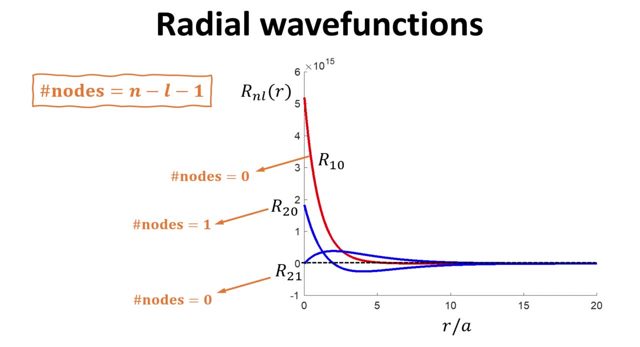 radial functions with l equals 0.. For n equals 1, we have only one radial function with l equals 0.. For n equals 3, we have three radial functions with l equals 0,, 1 and 2.. Let's plot these radial functions Here. we plot the radial functions for n equals 1 and 2.. 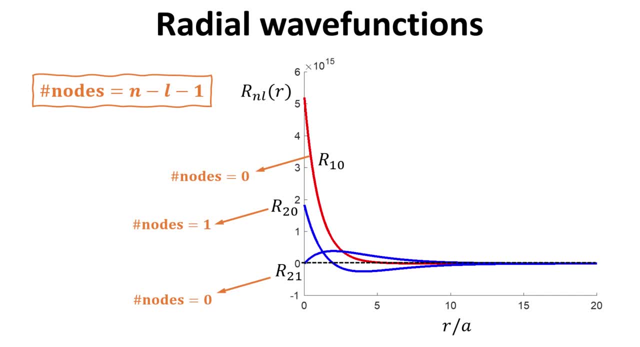 For the radial function r10, as given by the red curve. it has maximum at r, equals to 0, and decays exponentially with r. In other words, this wave function yields the largest probability of finding electron at the center of the proton. 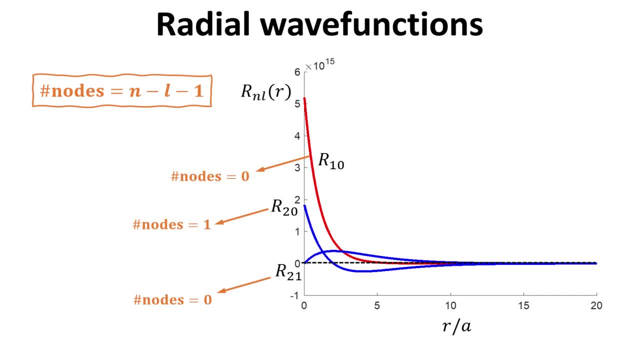 but with finite probability elsewhere outside the proton. For the radial function r20, it also has. the maximum at r equals 0. It decreases with r, then goes negative and slowly converge asymptotically to 0. Hence it intercepts the x-axis. once We call the number of nodes as the number of times it 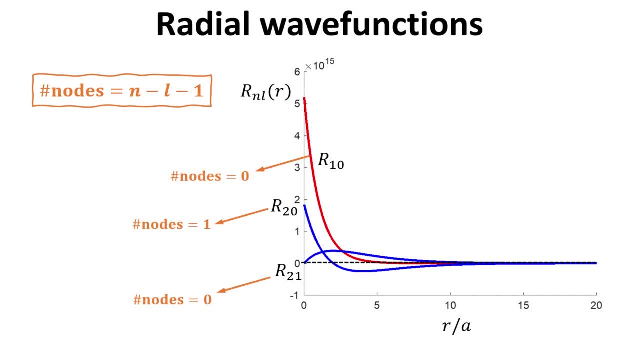 crosses the x-axis, which, in this case, is the number of times it crosses the x-axis. In fact, there is a simple formula that tells us what the number of nodes should be given by n minus l minus 1.. The radial function, r21,, on the other hand, 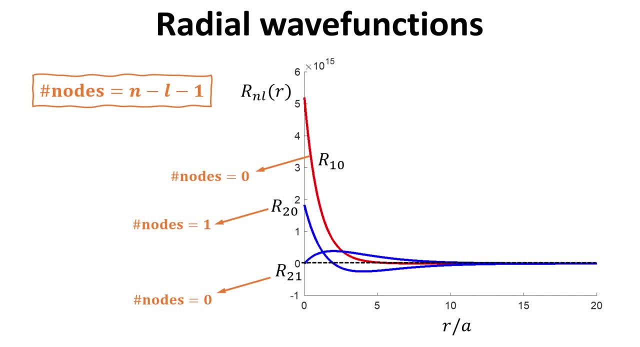 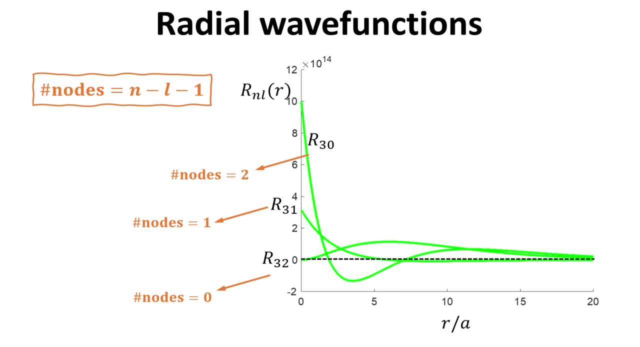 has zero probability at r equals 0.. Thus we see that the electron is not always at the center of the proton, as what one would expect classically. We can also similarly plot the radial functions. for the n equals 3 case, We have the functions r30,, r31, and r32. Again, one can count the number of nodes and check that. 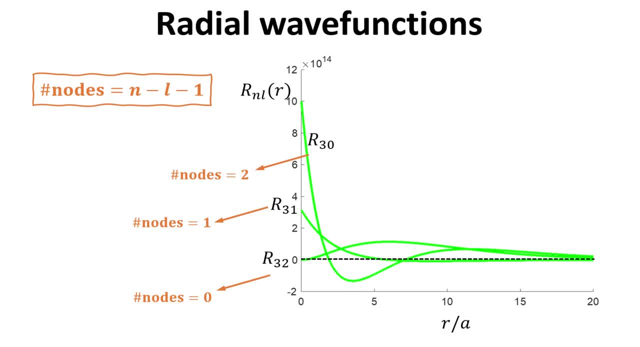 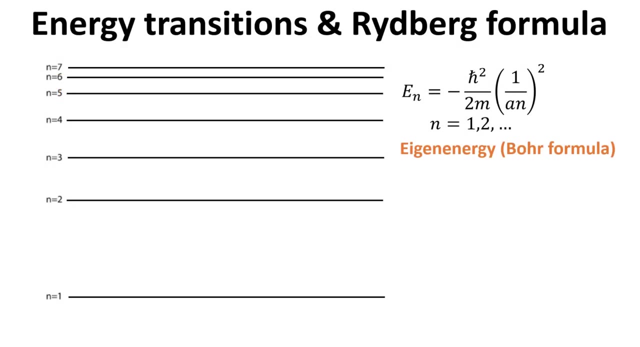 it is consistent with the formula as given. Qualitatively speaking, we see that the higher the index l, the more the wave functions spread out away from the center of the proton, out to larger r. All right, How about the eigenenergies? The energy spectrum of the electron is the same as the energy spectrum of the electron. The energy spectrum of the electron is the same as the energy spectrum of the electron. The energy spectrum of the electron is the same as the energy spectrum of the electron. 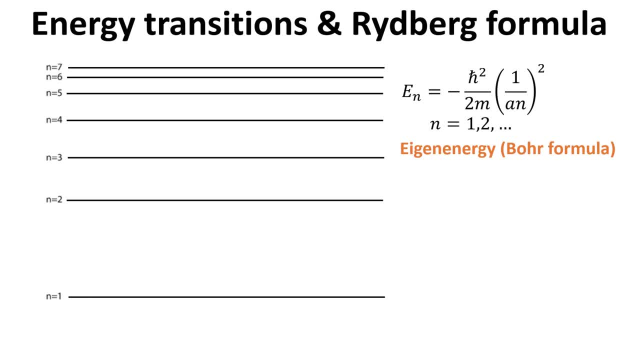 The energy spectrum of the electron and the hydrogen atom is given by the Bohr formula, and we plot here for energies corresponding to n equals to 1 to 7. The energy spacing decreases with increasing n. Electrons in the hydrogen atom can occupy any of these discrete energy levels. 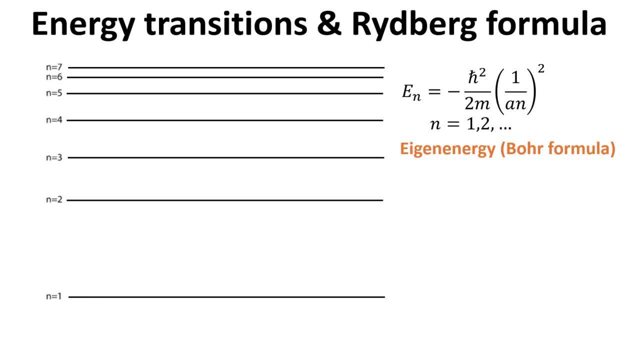 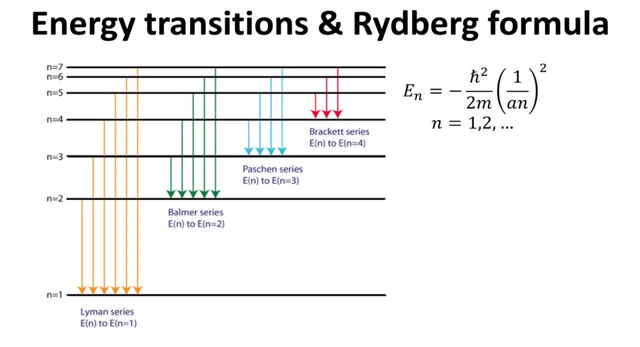 They transition from lower to higher energy level by absorbing a photon and vice versa by emitting a photon. The latter leads to distinct emission spectra for the hydrogen gas, which we have seen in previous videos. These emission spectra are described by different transition series. For example, the Lyman series described transitions from energy levels with n larger than 1 to n equals to 1.. 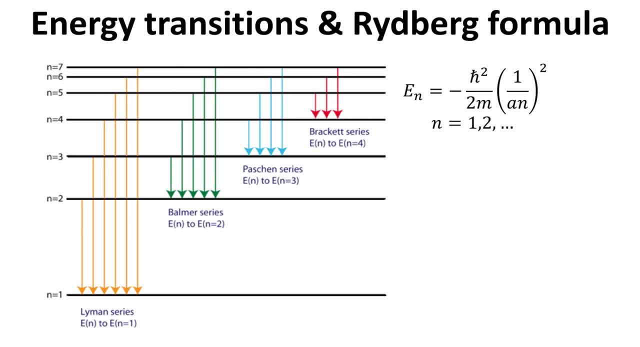 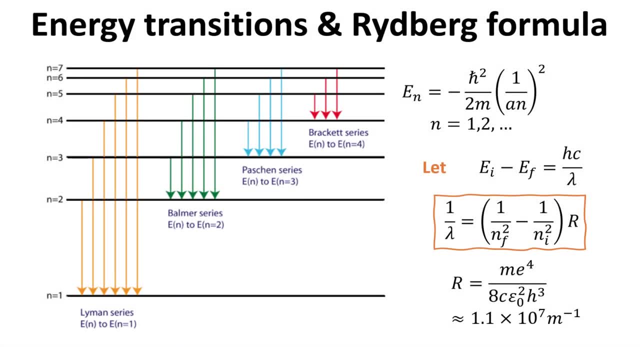 The Balmer series described transitions from energy levels with n larger than 2 to n equals to 2, and so on. Photons with wavelength lambda will be emitted when electrons descend from a higher energy level, EI, to a lower energy level, EF. 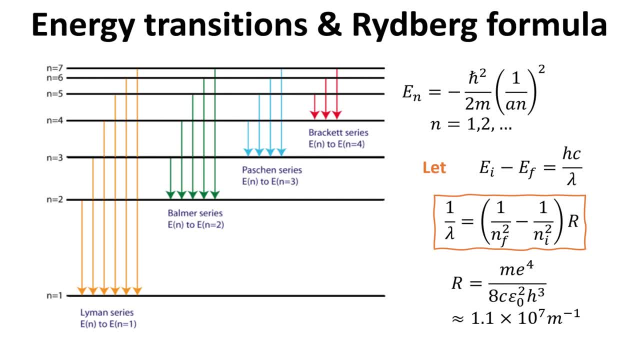 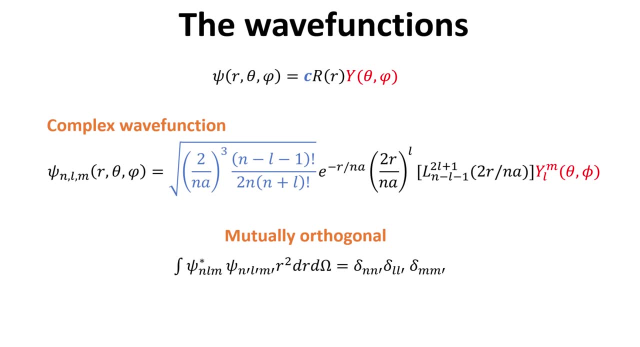 Lambda can be derived easily from the Bohr formula as shown in the orange box. The constant factor R is called the Rydberg constant and the formula is highlighted and called the Rydberg formula. The complete electron wavefunction is then given by the product of the radial function R. 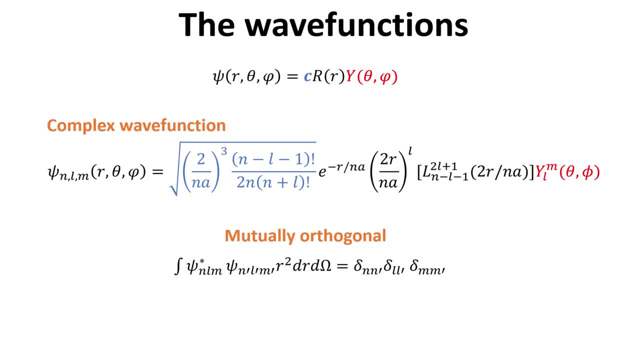 with the spherical harmonics Y, There will be a normalization constant for the function R, which we denote as C, whose expression is given in blue. The wavefunction is complex, since the spherical harmonics Y is complex. 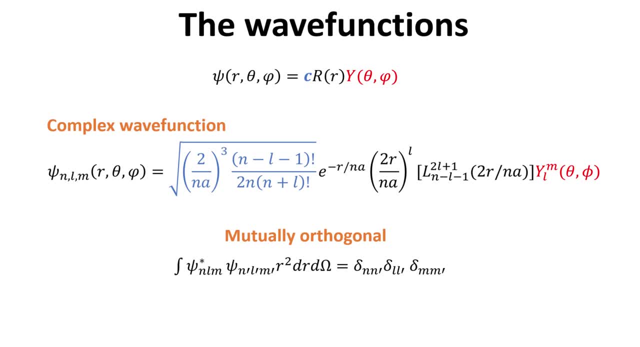 The atomic orbital wavefunction are indexed by three quantum numbers: n, l and m. These wavefunctions are mutually orthogonal, In other words their overlap with one another is zero, unless the three quantum numbers n, l, m are equal to n prime. 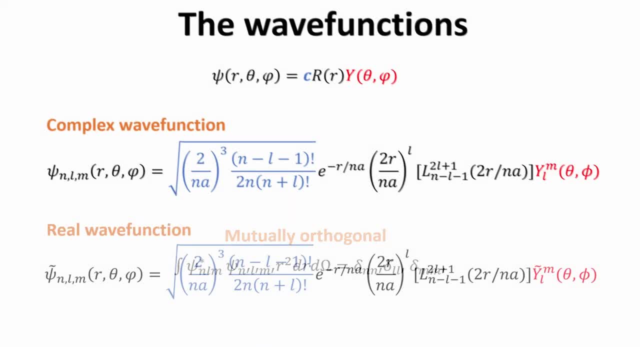 L prime and m prime respectively. However, through linear combinations of the complex spherical harmonics, we can construct a new set of real spherical harmonics. We have discussed how to construct real spherical harmonics in a previous video on spherical harmonics. In what follows, we shall discuss our visualization of these wavefunctions. 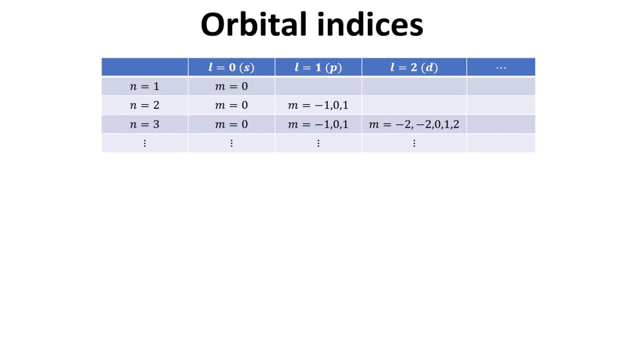 Before we proceed with the visualization of the orbital wavefunctions, let's remind ourselves again how the quantum numbers n, l and m are ordered. The quantum number n runs from 1,, 2,, 3 and so on. For each n, we have the quantum number l that runs from 0 to n-1.. 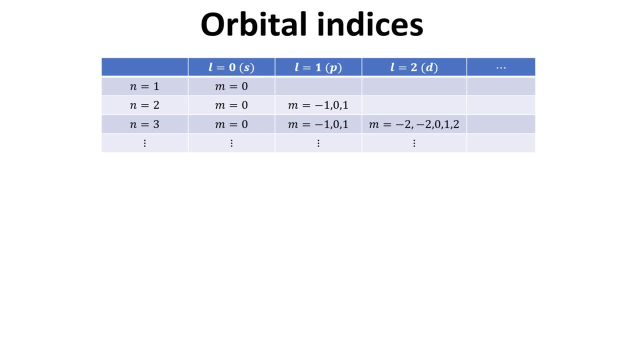 Lastly, for each l we have the quantum number m. that runs from minus l to plus l. Here we also adopt the common convention and denote the? l equals to zero orbital as S, the l equals to one orbital as P and the l equals to two orbital as d. 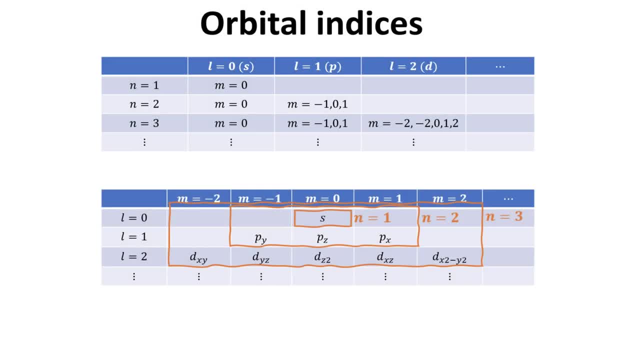 With a bit of reordering we arrive at the new table. For n equals to 1,, we have only one S orbital. For n equals to 2,, we have one S orbital and three P orbitals. For n equals 3,, we have one S orbital, three P orbitals and five d orbitals. 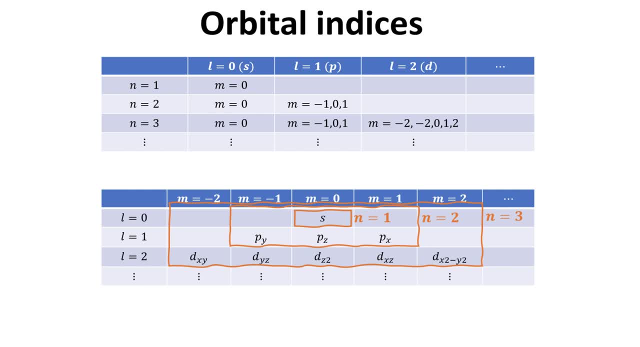 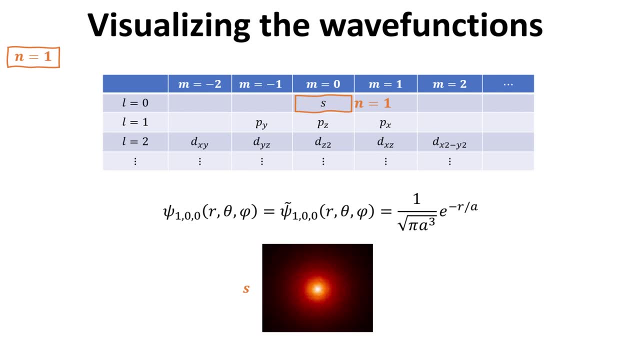 In what follows we shall visualize these different atomic orbitals. Let's start with the n equals to 1, which has only one s orbital. In this case the complex and real wavefunction has exactly the same form as shown. It is maximum at the center of the atom and decays exponentially with r, as depicted in. 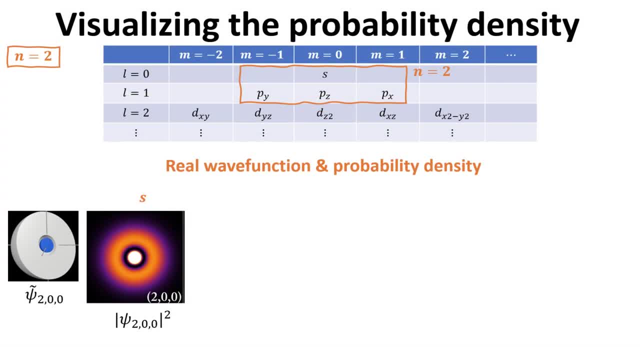 the image below. Next let's proceed to the n equals to 2.. In this case we have total of four orbitals: one s orbital and three p orbitals. In this case the wavefunctions are in general complex. 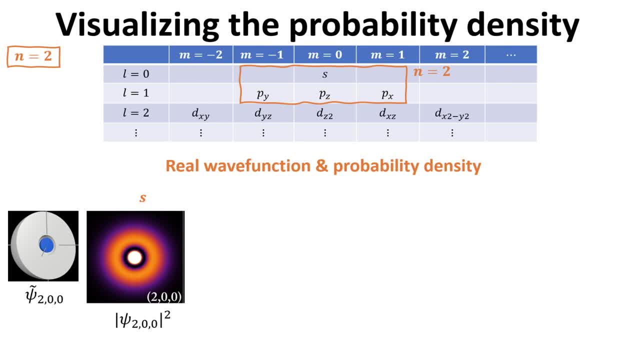 For the complex wavefunction we plot instead the probability density, which is modulus square of the wavefunction. This is shown in the red intensity figure where the brightness denote the magnitude of the probability. We see a large electron density in the core and also has a finite probability at some. 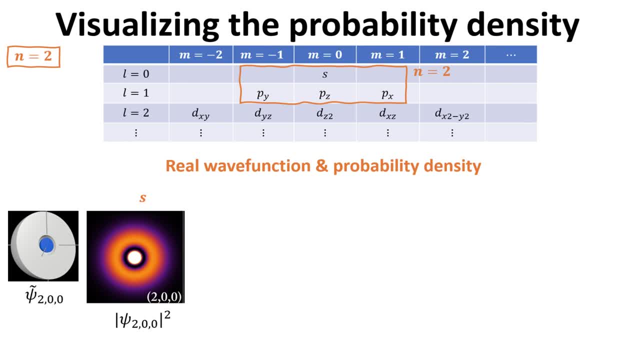 annulus ring In between the electron density is zero. This is a result of the fact that the radial wavefunction has a node. We can also plot the real wavefunction denoted by psi tilde. Here the sign of the real wavefunction is denoted by the two colors. 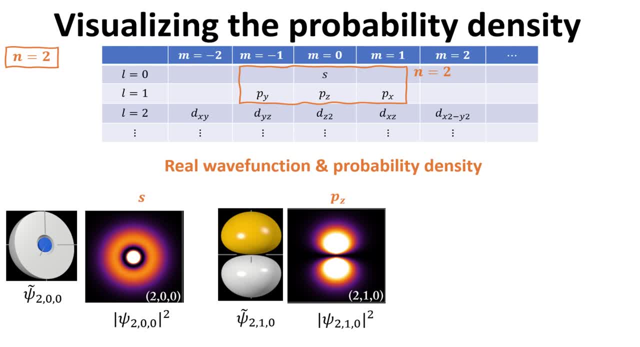 Next we look at the p z orbital. Here the sine of the real wavefunction is denoted by the two colors. Let's get a look at the p z orbital. It has a shape that like its real spherical harmonics we discussed in last video. 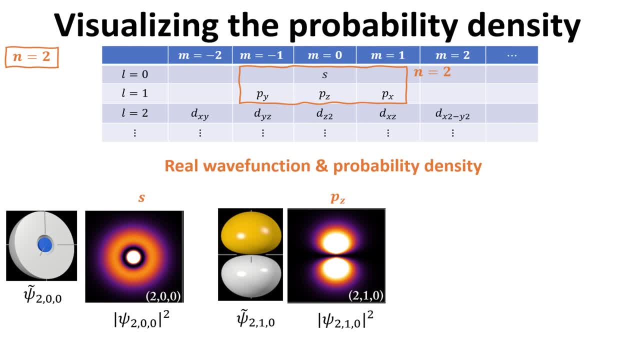 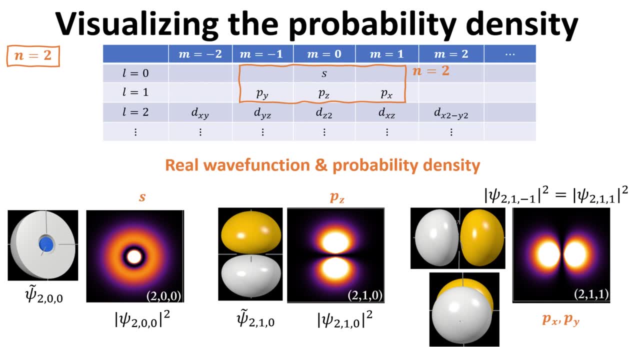 It has two lobes, with the lobe axis pointing along the z direction. Lastly, we visualize the p, x and p y orbitals. The real wavefunctions are like the p? z orbital, except that the lobe axis are now pointing along x and y respectively. 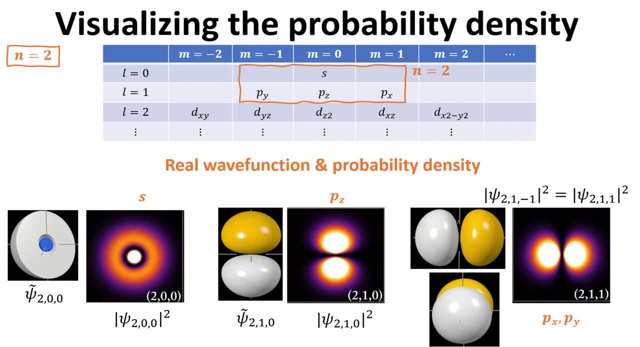 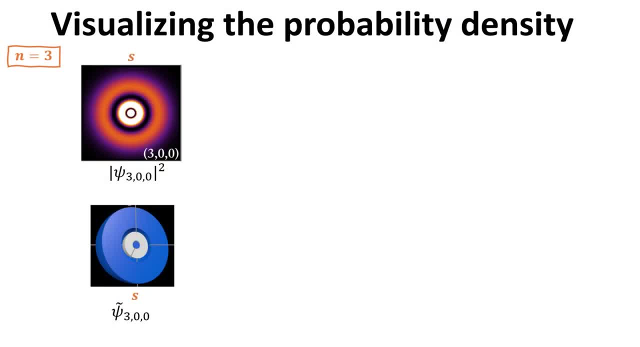 On the other hand, the modulus square of the complex wavefunctions p x and p y are now p-y are equal and is a torus shape lying on the x-y plane. Finally, let's look at the n equals to 3 case. We start with the s orbital Here. 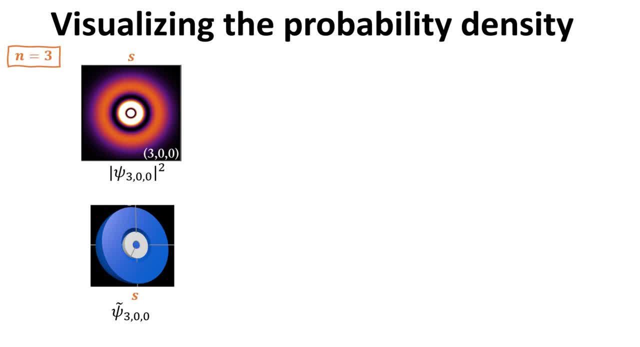 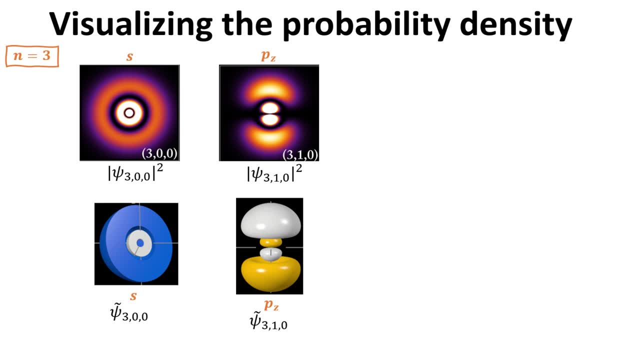 we see there are a total of two nodes along the radial direction, consistent with what we expect from the radial wave function. For the p-z orbital, we see a doubling of the number of lobes to 4.. The number of nodes along the radial direction is 1,, consistent with the radial wave function. 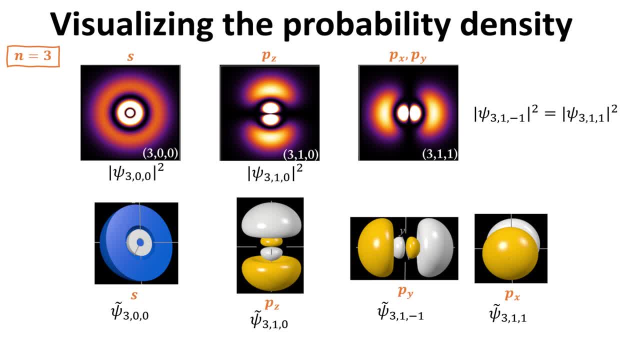 For the p-y and p-x real orbitals. they are similar, except that the lobe axis are pointing along the y and x axis respectively. The probability density, on the other hand, are equal and has the shape of an inner torus.